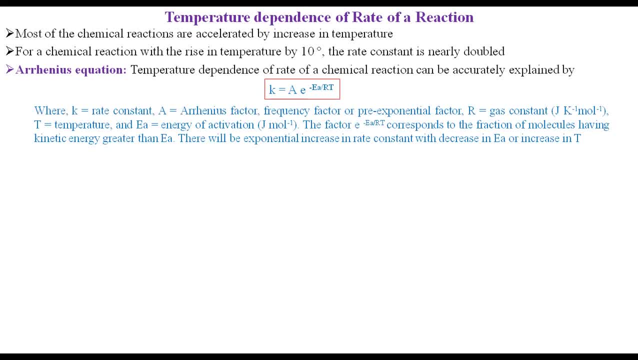 rate. constant A is Arrhenius factor, also called frequency factor or pre- exponential factor. R is gas, constant T is temperature and Ea is the energy of activation. The factor e power minus Ea upon RT corresponds to the fraction of molecules having kinetic energy greater than activation energy. This equation 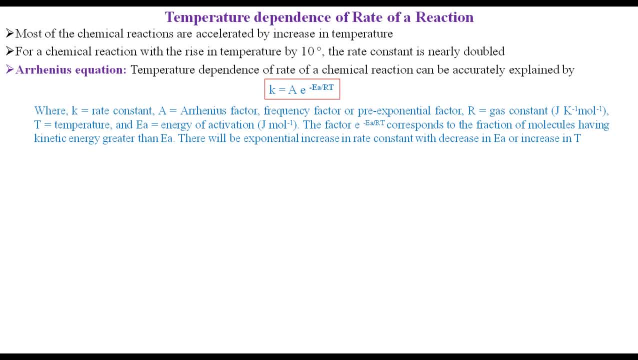 shows that there will be exponential increase in rate, constant with the decrease in energy, of activation or increase in temperature. Let us take a hypothetical reaction in which reactant A combines with reactant B to produce product P. According to the Arrhenius, A and B combine with each other to form an. 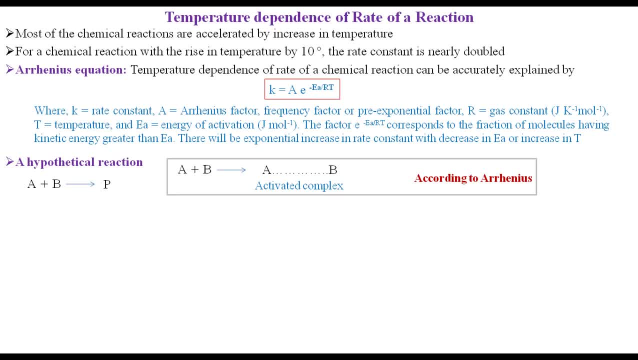 unstable intermediate called activated complex. It exists for a very short time and then breaks to form products. The energy profile diagram, which is a plot of potential energy versus reaction coordinate, can be shown as follows From this graph: energy of activation of a reaction is the energy. 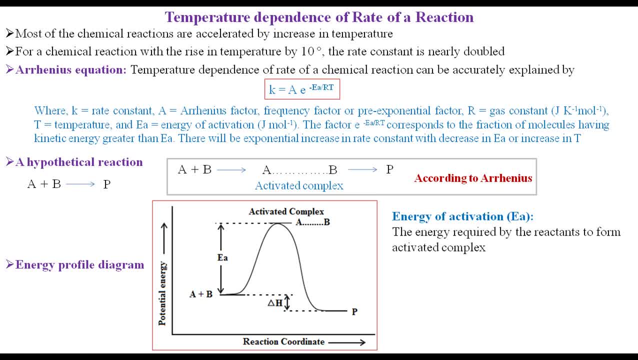 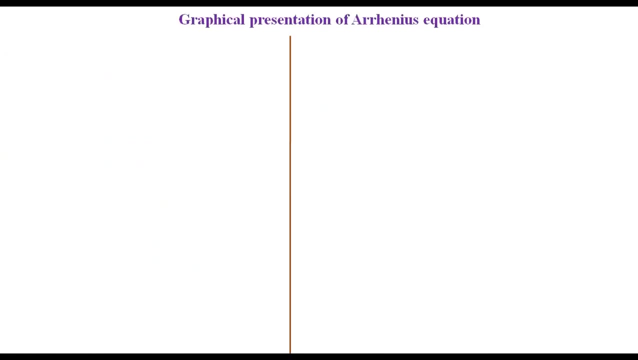 required by the reactants to form activated complex, or in other words, energy of activation of a reaction is the difference between the energy of activated complex and the reactant. Heat of reaction is the difference between the energy of product and the reactant. Graphical presentation of Arrhenius equation. We know that the Arrhenius equation 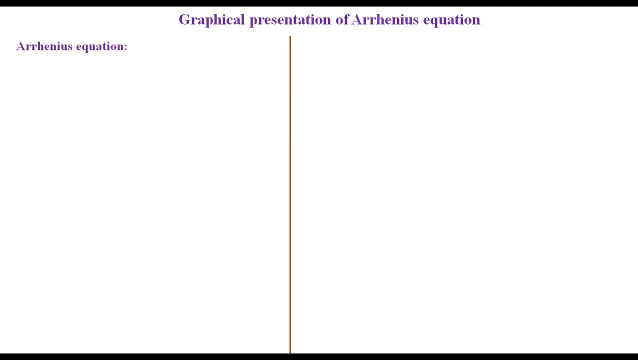 k is equal to A, e power minus Ea upon RT, where A and R are the constants For a particular reaction, Ea is also fixed. So if you plot rate constant against the temperature, we would get an exponential curve like this: This shows that the rate 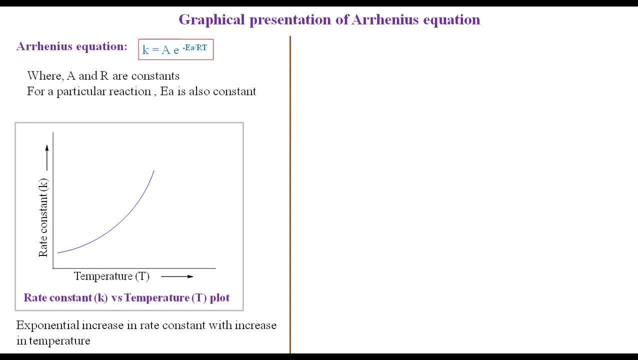 constant increases exponentially with the increasing temperature. If we take natural log of both the sides of Arrhenius equation, we will get: ln k is equal to ln A minus Ea upon RT. Rearranging this equation we will get the initial loss will result: ln k is equal to minus Ea upon RT plus ln A. 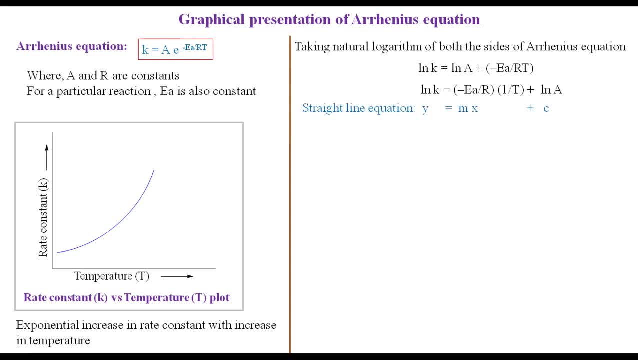 Comparision of this equation with the straight line. equation y is equal to mx plus C suggests that if we plot ln k against 1 upon T, we will get a straight line with. the slope is equal to Ea on R and the intercept is equal to GN. k times k times b equals equalto convergence of the Real deserve totalol minus εt. 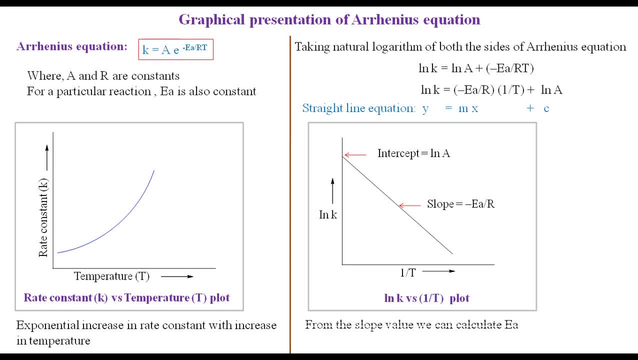 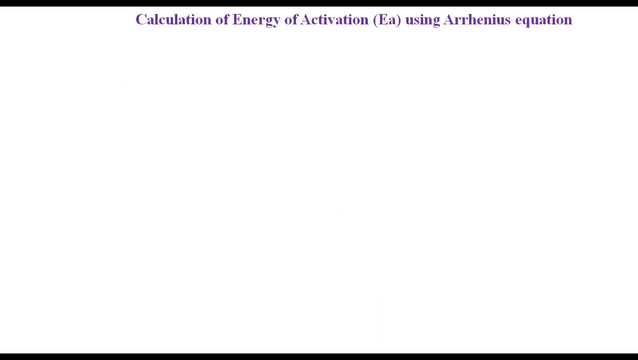 LnA. Thus from the slope we can calculate the energy of activation. Calculation of energy of activation, Ea using Arrhenius equation. Arrhenius equation for a particular reaction at two different temperature, T1 and T2, can be written like: as K1 is equal to 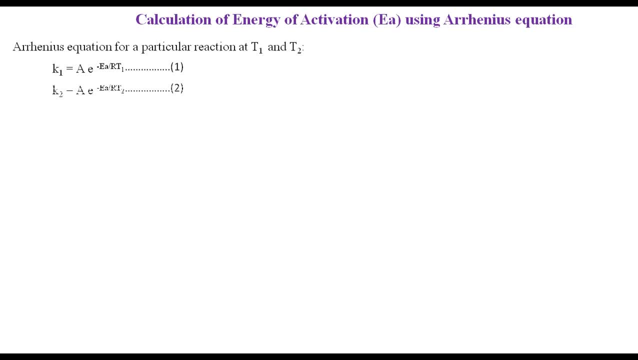 A into E power minus Ea upon Rt1.. K2 is equal to A into E power minus Ea upon Rt2.. Taking natural log of both the reactions will result: LnK1 is equal to LnA minus Ea upon Rt1.. LnK2 is equal to LnA minus Ea upon Rt2.. Subtracting equation number 3 from: 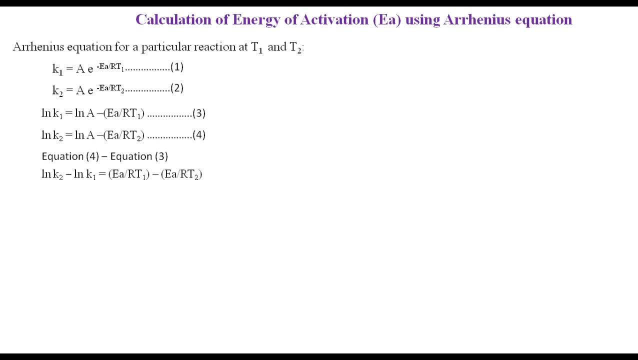 equation 2.. We will get: LnK2 minus LnK1 is equal to Ea upon Rt1 minus Ea upon Rt2.. Or we can write: LnK2 upon K1 is equal to Ea upon R1 upon T1 minus 1 upon T2.. We can also write 2.303 log K2 upon K1.